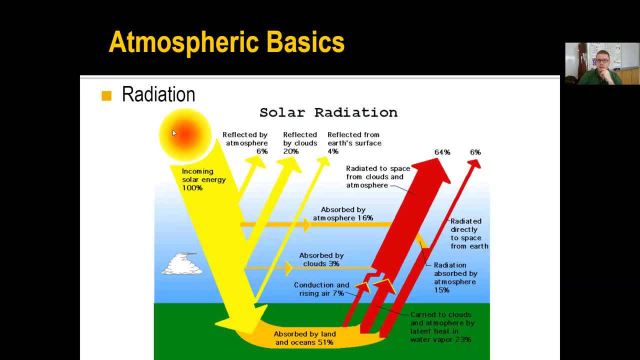 to kind of taken. so we start with the sun. incoming solar radiation from the sun, Some of it is reflected by the atmosphere, Some of it is reflected by the clouds, Some of it is reflected by the earth's surface. The larger majority of it- 51% of the Earth's energy, the sun's energy- is absorbed by the land and by oceans. 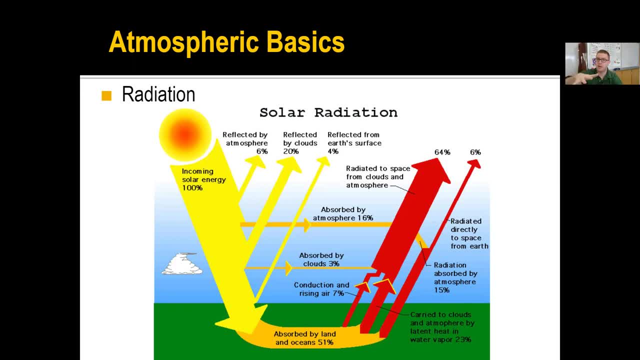 What happens then? Well, you know, it heats up, And then some of that energy is then radiated back into space, kind of like our light bulb does. Once we turn it on, it warms up and that heat starts coming off it. 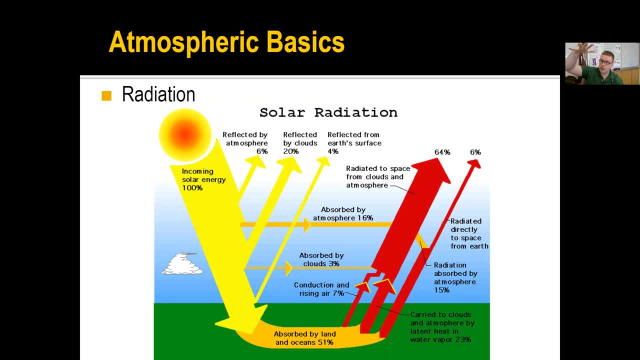 Same thing. We heat the ground from the sun. The heat is going to kind of radiate back up. 64% of it goes back to space. There you go, It goes back to space. Some of it goes directly back to space. 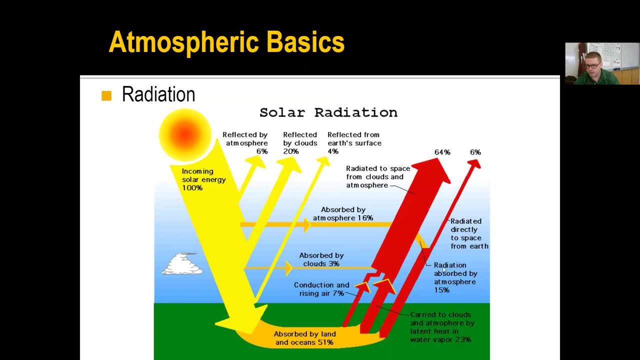 But then this little bit right here that's really interesting is that 15% of it warms the atmosphere because it's absorbed by the atmosphere. Different chemicals in our atmosphere, like water vapor, carbon dioxide, does a really good job kind of absorbing that extra radiated heat coming back up off the surface of the planet. 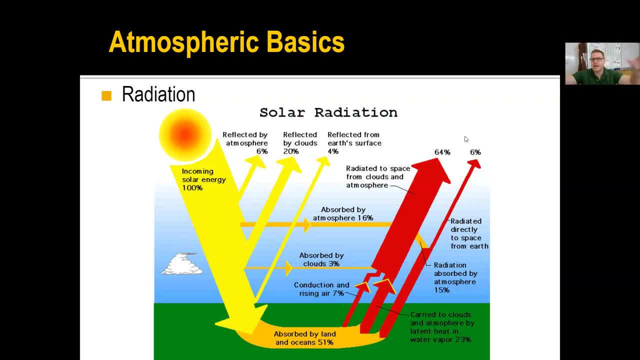 That keeps our planet warm, almost like a blanket around the entire planet Because of, you know, that extra cloud cover or that extra carbon dioxide or water vapor in the atmosphere. If you didn't notice this, sometimes at nighttime, when it's dark, no sun, and if it's a clear sky, it feels way colder than some nights that you know have cloud cover around the same temperature. 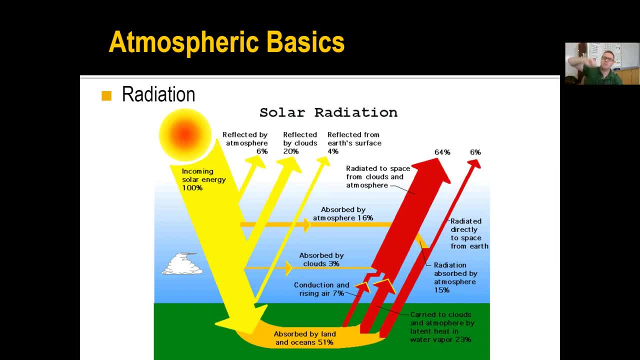 It's because that radiated energy from the surface it's escaping back out into space. There's no blast, It's just a blanket in that section. So cloud cover water vapor does a really good job, helping to insulate us down here at the surface from getting a little too cold sometimes at night. 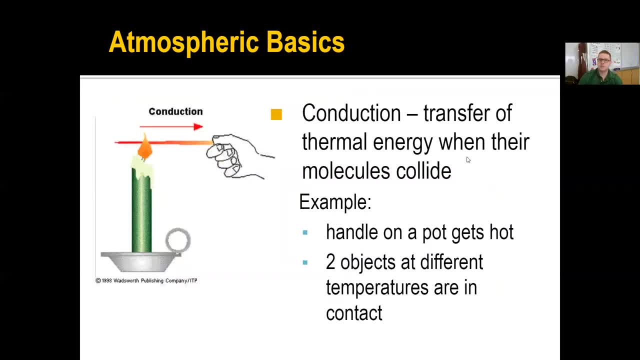 That's the first type. Second type is called conduction. This is the transfer of energy when molecules collide into each other. If you think about heating like a water pot on your stove, the pot itself has a handle attached to it. That water is going to boil and do its thing, but then the pot itself is going to warm up. 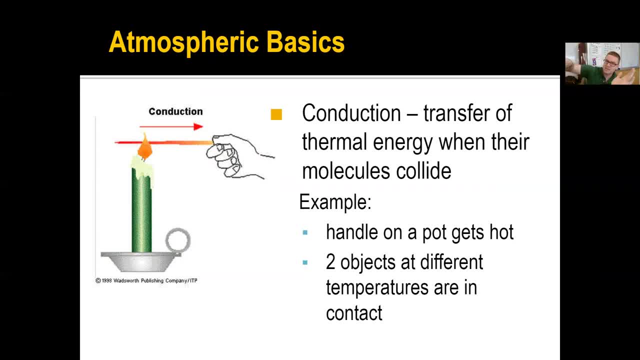 And then eventually that heat will be conducted to the handle. almost. like you know, a conductor, like electricity, Metal's a good conductor for heat also. So if I heat up like the source, like the pot here, that temperature will eventually work its way to the handle and that handle will heat up. 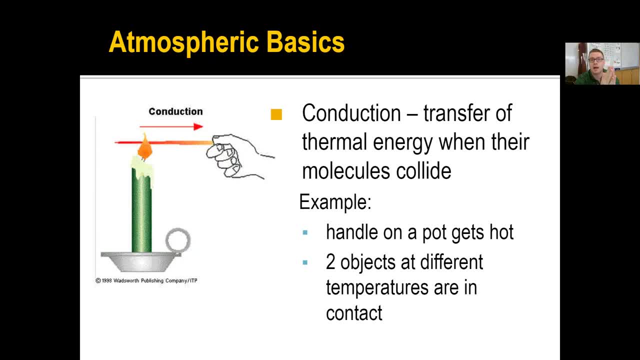 That's why sometimes you have two objects at different temperatures even though they're in contact with each other. Sometimes it takes a little longer for that second bit like that handle to warm up. That's why most pots they have They have kind of like an insulated handle so you don't burn your hand when you're boiling water. 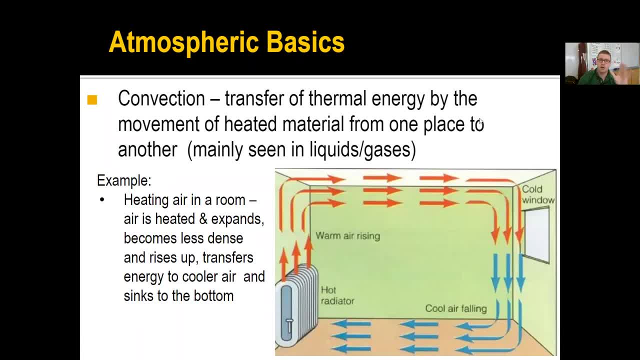 That's conduction, The third type we've spoken about before. we were talking about the mantle, We were talking about convection and plate tectonics. It's the transfer of thermal energy by heated material moving from one place to another. 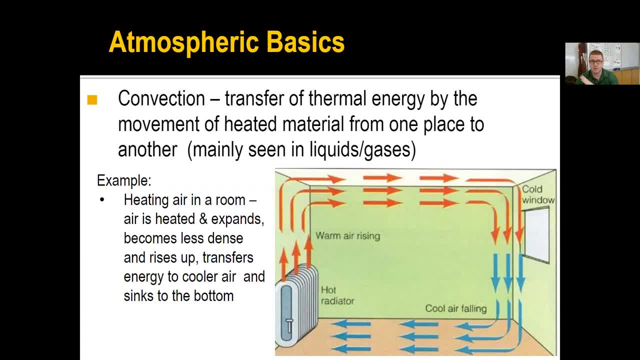 And it has to do with, you know, heated material being less dense, being able to rise up in the atmosphere and colder temperature material being more dense and a little sink. Then we get this rising motion, movement and this heating sinking motion and movement. 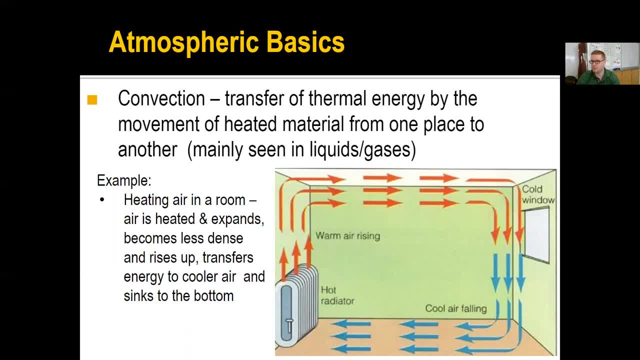 So it's this difference in high temperatures and low temperatures and high densities and low densities that can cause kind of this rotation in our atmosphere, And we'll come back to this a little bit. We're talking about areas of high pressure, low pressure, precipitation, fair weather in a later section. 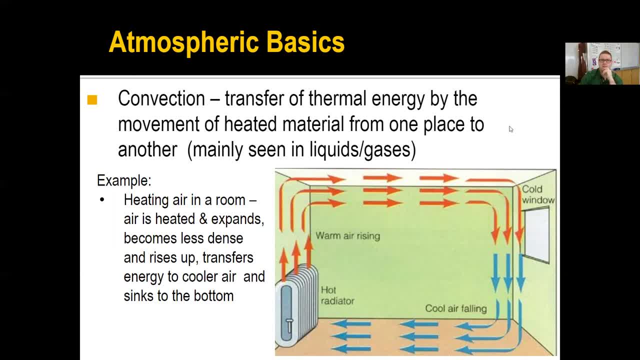 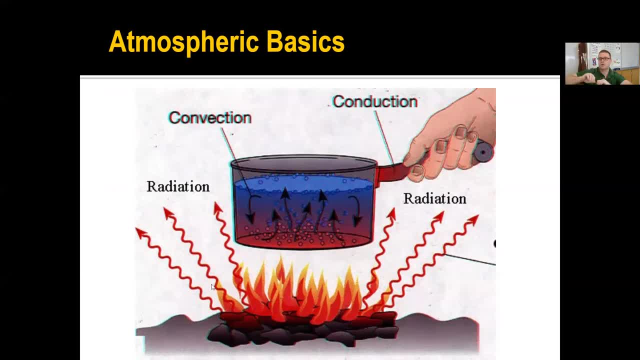 Just know convection. it's a circular motion because of temperature And density differences. Here's a great picture that shows all of this in motion. We have radiation from that heat source coming off of this fire. We have convection going on in this pot. 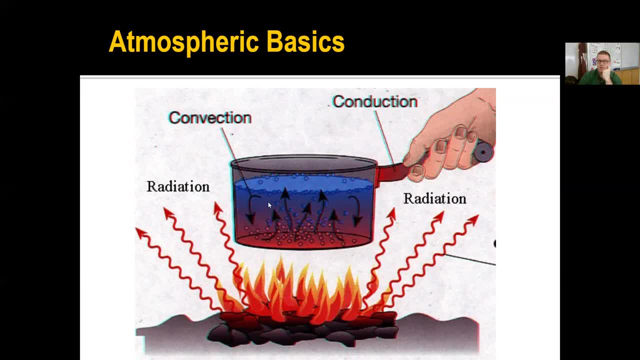 As warm molecules increase their temperature, they're going to rise to the top, They'll cool a little bit and they'll sink, causing this circular convection in the pot Conduction. we have that metal handle touching the base of the pot. 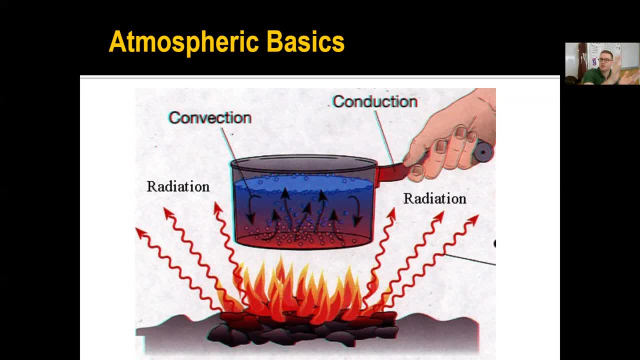 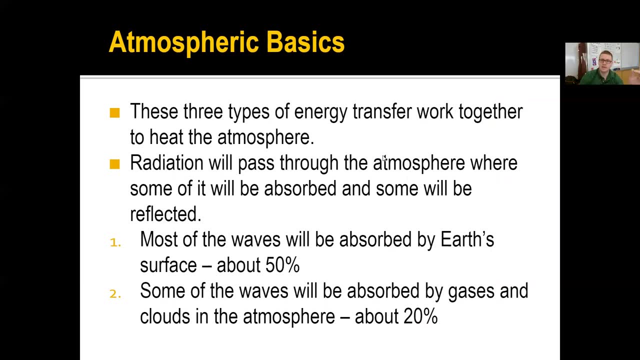 That's going to warm up a little slower, As that heat Conducts through that material. So radiation convection, conduction, they all work together to heat our atmosphere. Now, like I said at the beginning, radiation will pass through the atmosphere. 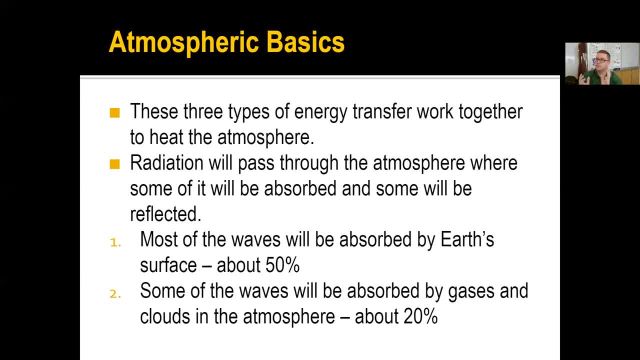 Some of it reflects back into space, Some of it makes it through and absorbed by the surface of the planet. Of these waves that are absorbed, it radiates back up. Some of the radiation coming back up in the atmosphere, Somewhere between 16 and 20%, is going to be reabsorbed by the atmosphere, giving us that greenhouse effect. 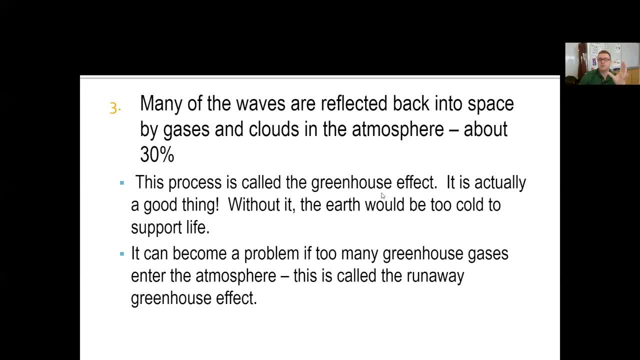 That's a good thing. Without the greenhouse effect, Earth would be too cold to support life And you know we wouldn't be here playing this game. Now. the issue is, if we have too many greenhouse gases in the atmosphere, it can get warmer and warmer, and warmer and, you know, might hit a point where it's just out of control. 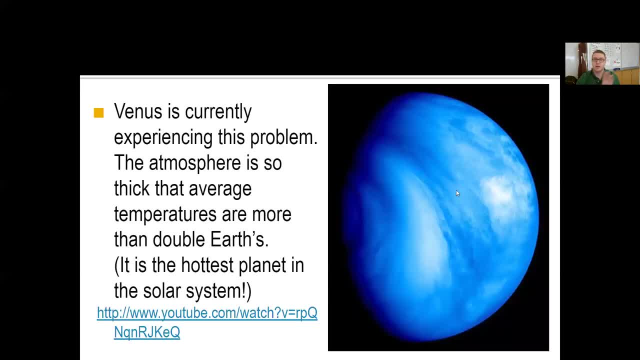 We call that a runaway greenhouse effect. You see this with. you know, one of our neighbors in our solar system, Venus, is experiencing a runaway greenhouse effect. The atmosphere is so thick that the average temperature on Venus is considerably more than double that of Earth. 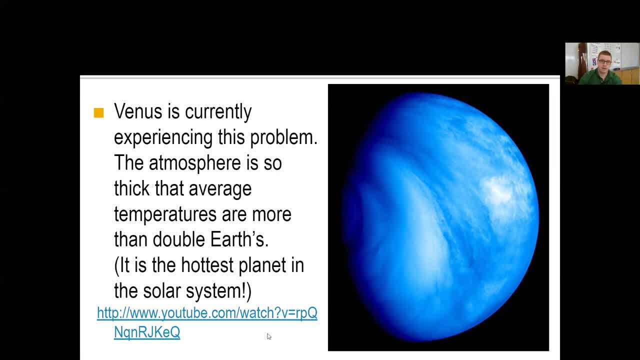 It's one of the hottest planets in our solar system. There's a URL link in our slides here. I encourage you to click on. It'll take you to a video that discusses Venus's greenhouse effect and how it's, you know, causing some problems with Venus. 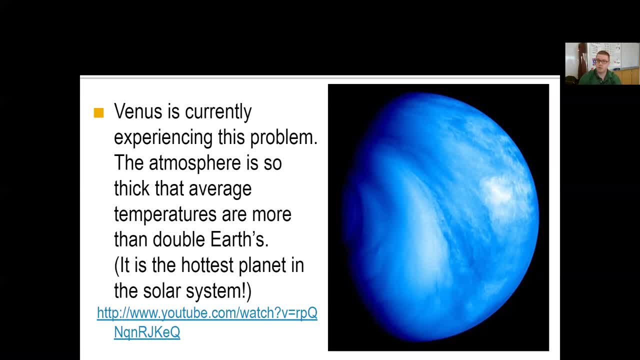 Now there is some studies out there that feel that Venus at one point in time in the past was habitable, and then stuff occurred that you know eventually led to a runaway greenhouse effect. Could it have been an abnormal amount of volcanic eruptions possible? 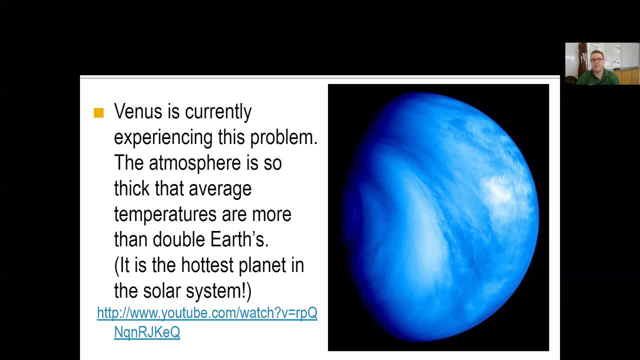 That is one way of getting a lot of carbon dioxide into the atmosphere. There are other, you know ways to kind of like increase the amount of water vapor in the atmosphere too. So I encourage you to watch that video, Seeing what's going on with Venus and just learning a little bit more about that. 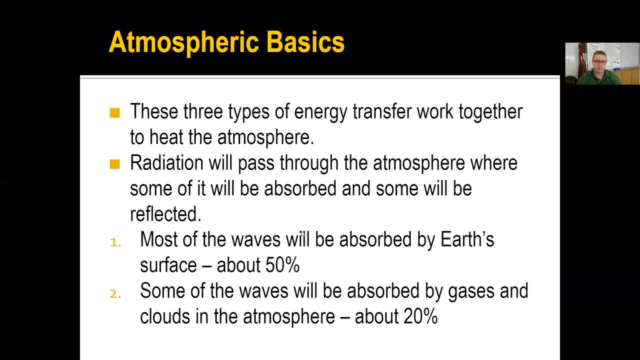 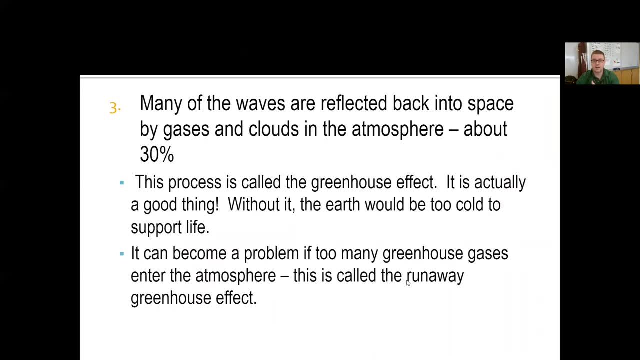 So, in summary, again let's rewind here. We have radiation convection, conduction and the greenhouse effect being kind of powered by the radiation from Earth's surface. That energy is being absorbed by the atmosphere, keeps us warm, keeps us, you know, from actually being able to support life on this planet, which is a good thing.